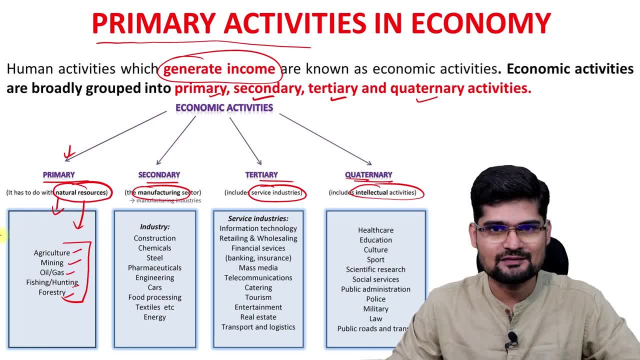 out the natural resources, which is basically primary activities, which we are going to learn in details in this session, And industry, which is basically construction, chemical, steel, pharmaceuticals and several others. These are secondary activities. Then comes the service industry. And now, as we know, during the lockdown, during the pandemic, 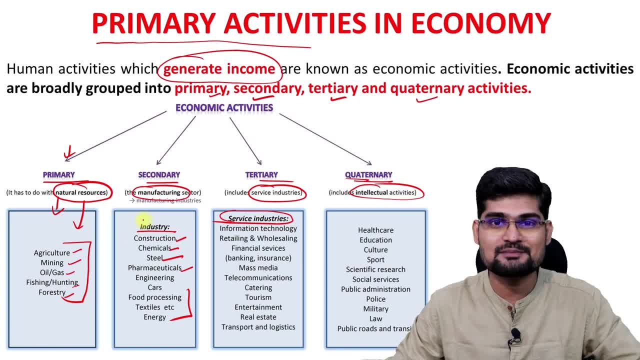 the service industry is what we were all dependent upon for the doorstep delivery and several other services, So we know that it is based on IT, information technology, retailing and wholesaling, financial services, mass media, telecommunications, tourism, entertainment, real estate, several. 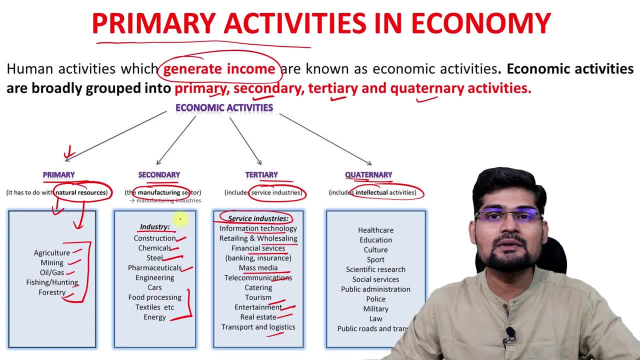 services that we get, From entertainment to the food industry, from the apparels to other. you know several other different kinds of industries. Remember, it's all tertiary. Then comes quaternary activities, For example healthcare, education, culture, sport, scientific. 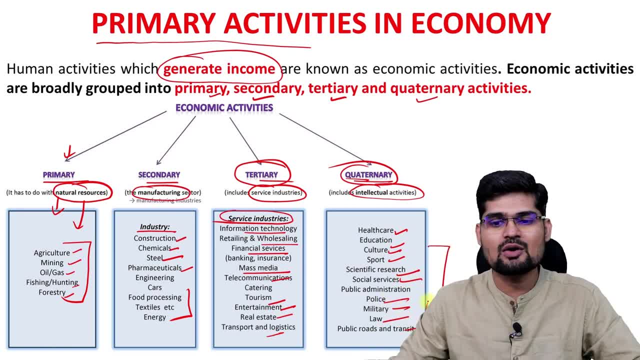 services, police, military law, public roads and transit. All these things are part of quaternary activities. Now, the entire economy is built on the four pillars, out of which we are going to learn about the first pillar, that is the primary activity. Now, when we say primary, 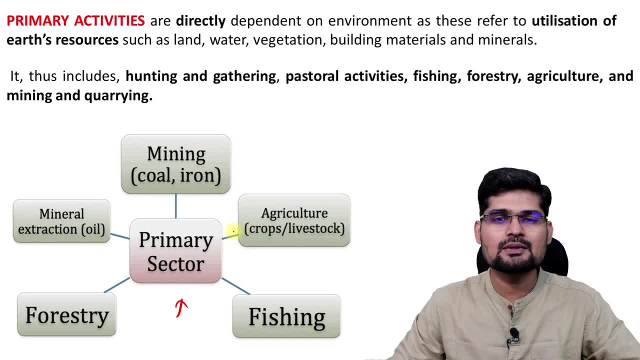 activities. this flow diagram is one thing which you can remember easily. So primary sector is based on mining, agriculture, fishing, forestry, mineral extraction. All these things are the major pivots of primary sector of economy, Primarily importantly, understood as the utilization of earths or natural resources. 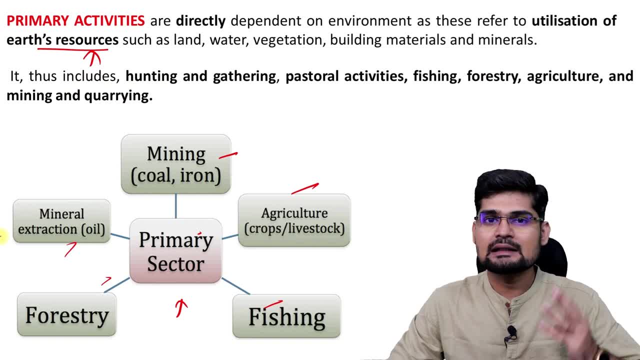 Right. So primary activity. whenever you hear the word should be natural resources coming to your mind. So land, water, vegetation, building materials and minerals occupy the major attributes of primary activities in our economy. Hunting and gathering, pastoral activity, fishing, forestry, agriculture, mining and quarrying- These things have been 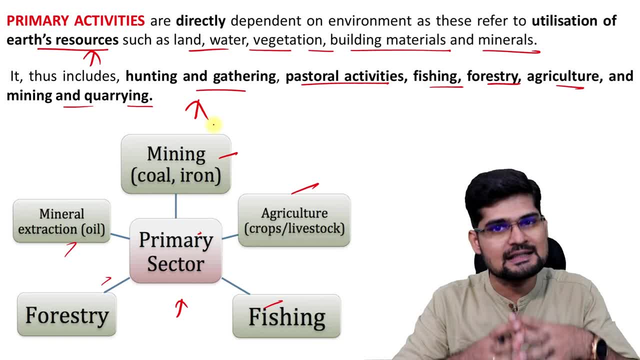 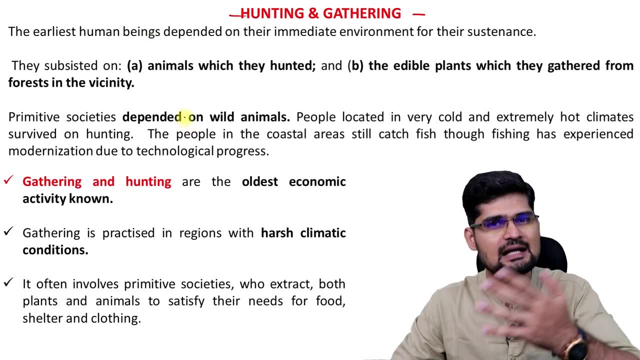 part of the primary sector of economy since its inception, Right. So now lets begin with the first one, that is, hunting and gathering, and then gradually go to the mining, fishing agriculture and its subtypes, Animals which were hunted and the plants which 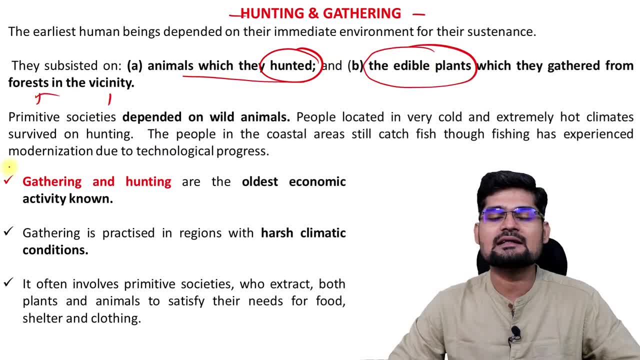 were edible. they were gathered from the forests in vicinity under hunting and gathering. It was the most primitive form of economic activity that we say. So gathering and hunting is the oldest economic activity, as we know, And normally in different conditions in 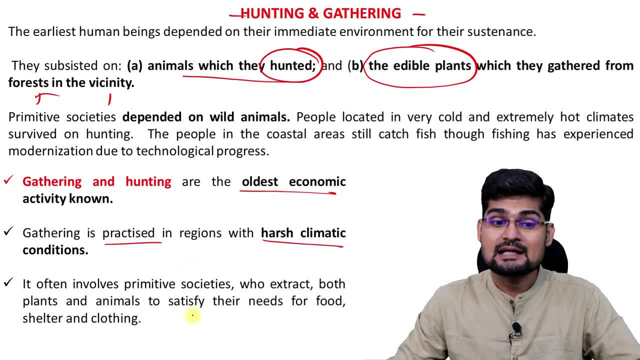 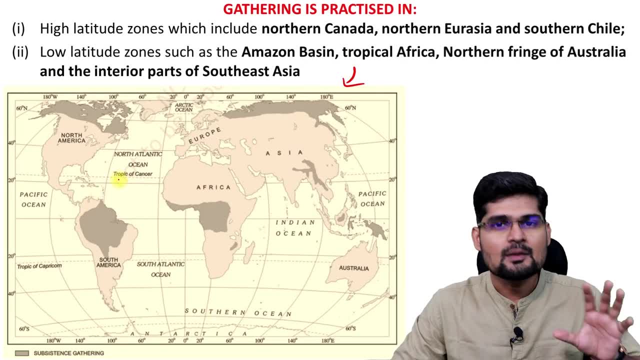 forested areas, in harsh climatic conditions, these were practiced. Gathering is still practiced in many societies. Many exclusions do not exist, so gathering is practiced where, if you observe, this is the world map and you can pause the video and also look into the world map, or you can get a world map and mark these areas in different. 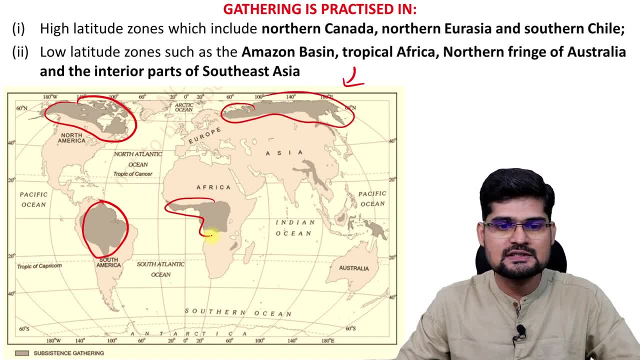 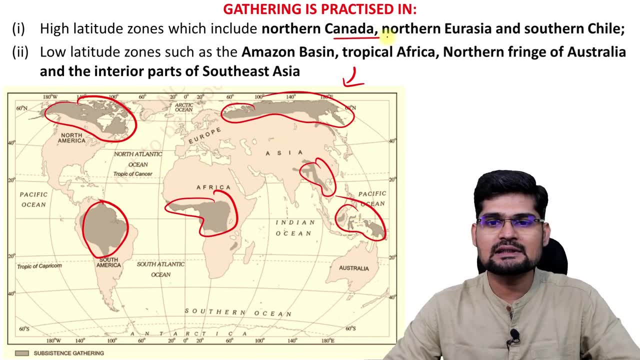 continents where you still have these areas, which is, dark areas on the map, where you see hunting and gathering still prevalent, so majorly gathering. if you observe northern canada, northern eurasia, southern chile, this is where you observe all the locations on the map: amazon basin, tropical africa. 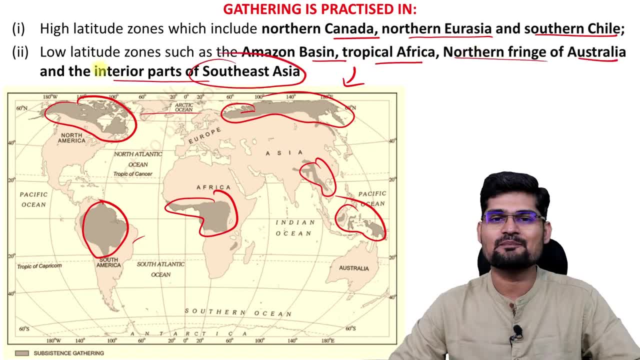 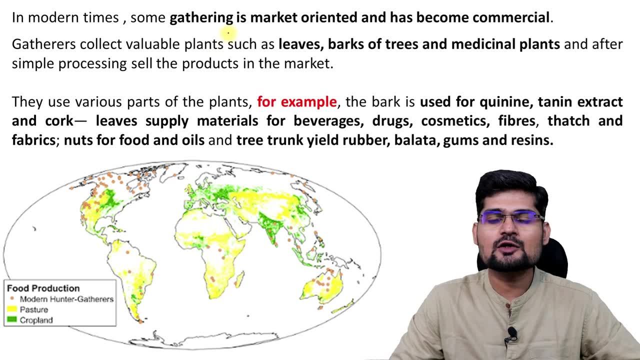 northern fringe of australia and interior parts of southeast asia. this is the world distribution of hunting and gathering in present times. then, in modern times, remember, gathering has occupied a commercial base as well. how, remember, we are collecting leaves, bark of trees and medicinal plants for so many commercial purposes in the market right. so now this gathering has become 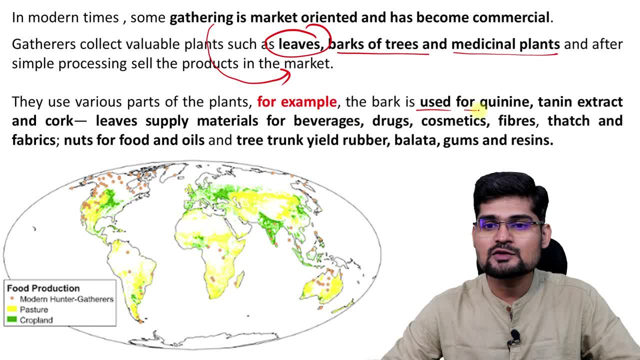 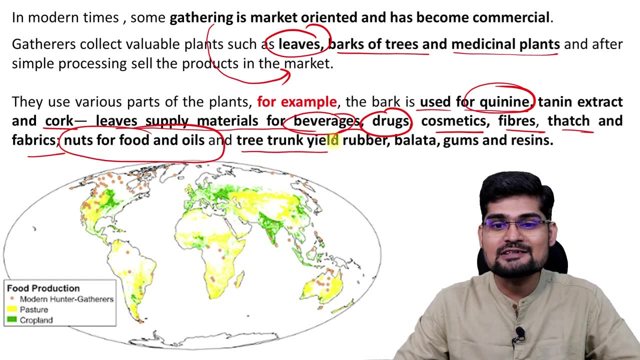 market oriented as well. for example, the bark used for quinine- remember, this is a cure for malaria- tannin extracts and cork leaves, supply materials for beverages, drugs, cosmetics, fibers, patch fabrics, nuts for food and oil, and then tree trunk yield, rubber, belata, gums and raisins. so we all know that this. 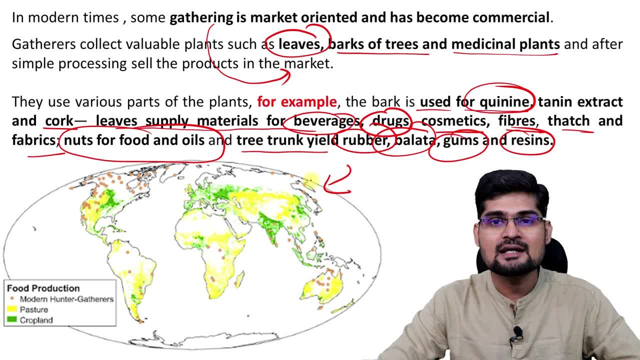 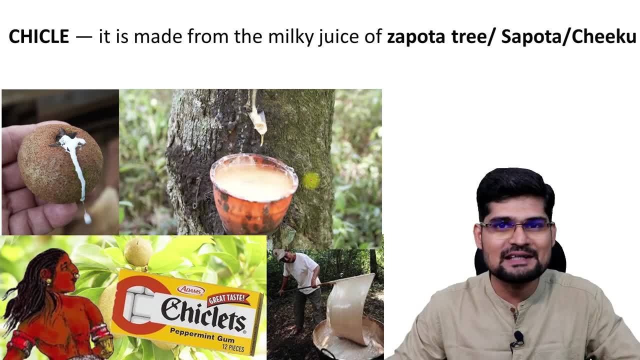 is prevalent across the world. these gathering activities are used for commercial purposes for so many examples, as we see here. right. so one of the example in almost your everyday life: if you are fond of eating chiclets, right? or the chewing gums, it is made from the milky juice of. 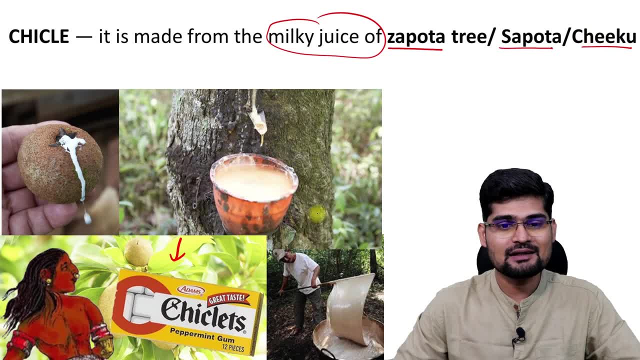 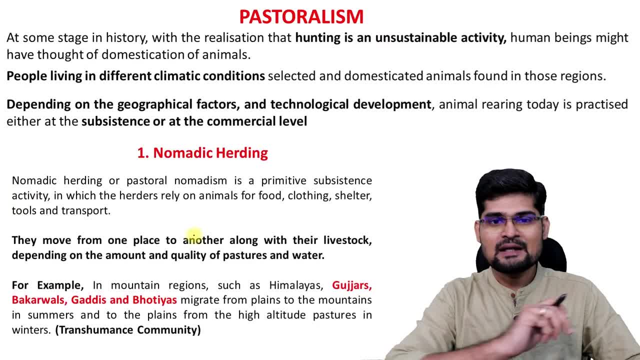 of zanthoxylum and it is made from the milky juice of zanthoxylum and it is made from the milky juice. often i have seen people mixed actually in many of these activity and event venticium in their game aspects. flipping went almost 100 years ago and after market genius. scientists actually started to collect. so this year, 신평 Το coraz swimming activity is visible comen expertise in. among the 70 Asian countries with domestic infestation, animals all have dark, hearty and keen disease. I whereby these amazed people. hence the learning activities. 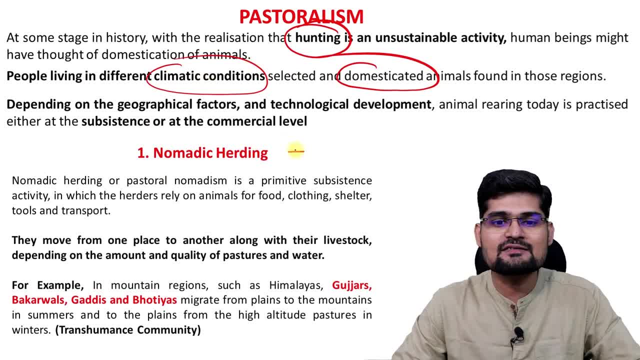 is domestication of animals, so under which you have several types of pastoralism. one of them is nomadic herding, and it is based on what? it is based on geographical factors, technological development. animal rearing today is practiced in several areas, from subsistence to commercial. 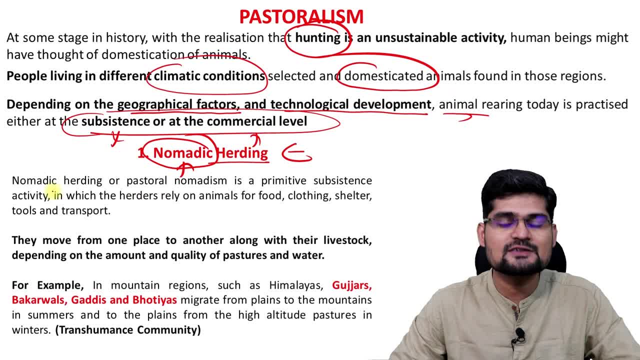 levels. so first of all, let's look into nomadic herding. the word itself is nomadic, so what is there? nomadic herders do what they move from place to place. it is one of the primitive type of subsistence right. so, for example, in India, if you want to observe, the community is living in. 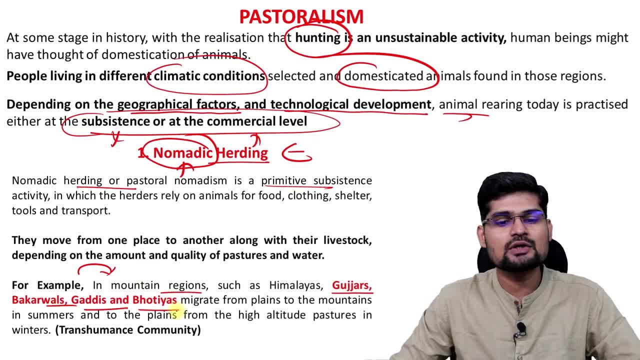 mountain regions like Gujjars, Bakarwals, Gaddis, Bhotiyas. these migrate from different areas, from lower foothills plains to the mountains. in summer, when the snow melt, they go to those valleys with their herds cattles to feed them for the season. this is also called transhumans community, so they 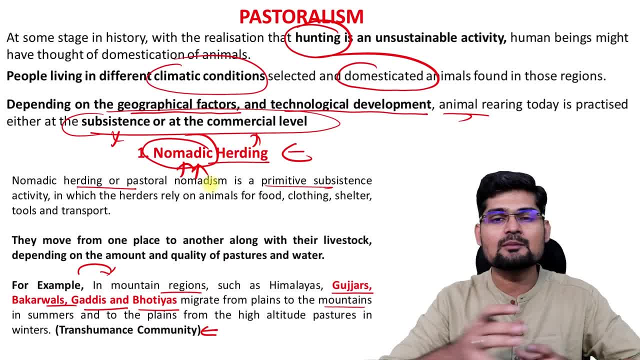 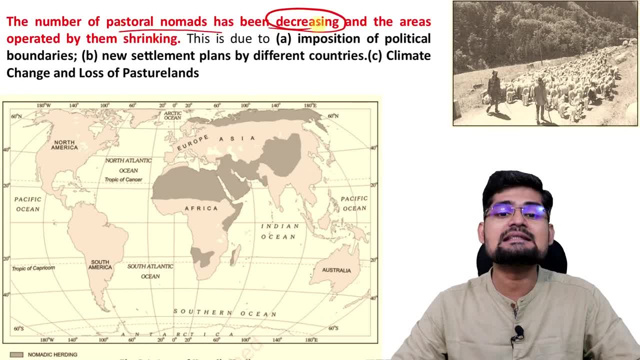 are not settlers at one location but they keep fluctuating, moving in the seasons, so that is part of nomadic herding. then number of pastoral nomads have been decreasing across the world. that is one important thing to understand and the reasons for that is imposition of political boundaries. 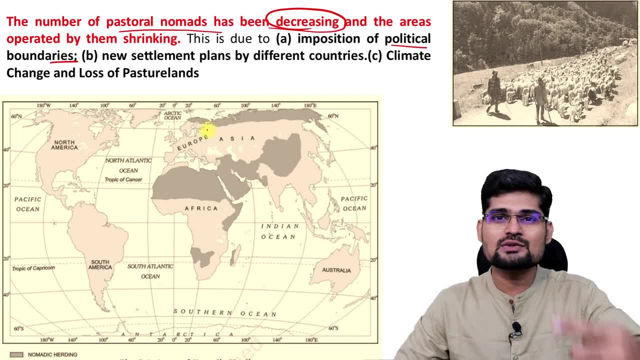 lots of political changes have happened. so one region to the other. if there is a boundary in between, if you are crossing two states, you have to go. it's very difficult. second is new settlement plans. development is coming up, so newer areas are taken up for the settlements, for developmental 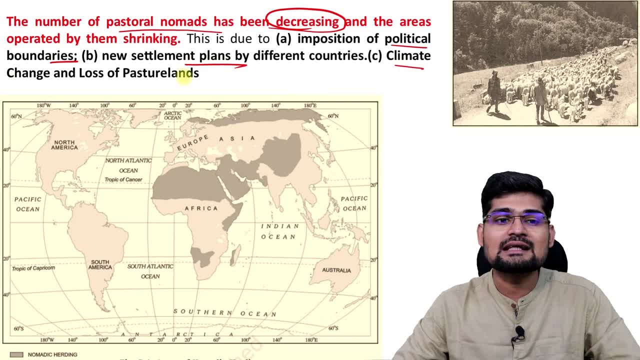 activities so that also hinders in this. and then, third one is the climate change and loss of natural lands. this is the recent phenomenon that has started happening in himalayan region, as well as different mountain regions of the world facing climate change. so if you observe this, dark portions- 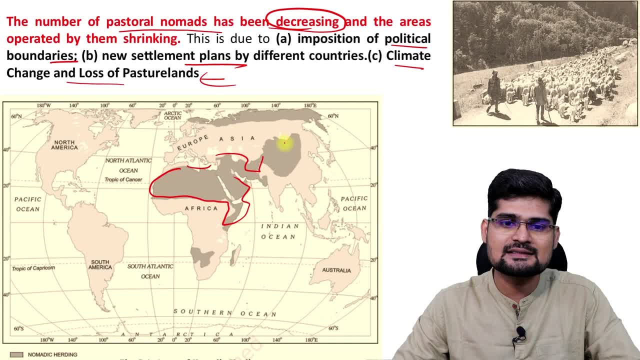 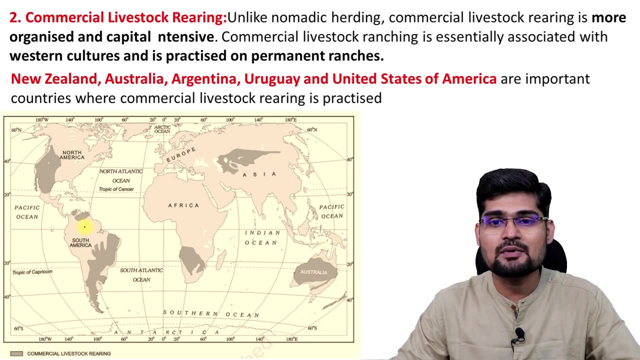 on the map here these areas of africa, middle east, central asia, north asia, right and northern tip here, and also some portions in southern parts of africa and madagascar, you find the concentration of these nomadic herders. then comes commercial level of livestock rearing. now this is very important. 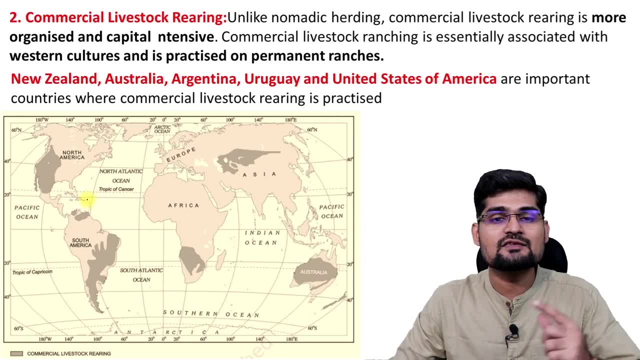 because it's commercial. it means people are not able to live in a place where there is no animal for the commerce, right. so it becomes capital intensive, right. that's really important and it is organized now. here is important point to remember that it is practiced on permanent. 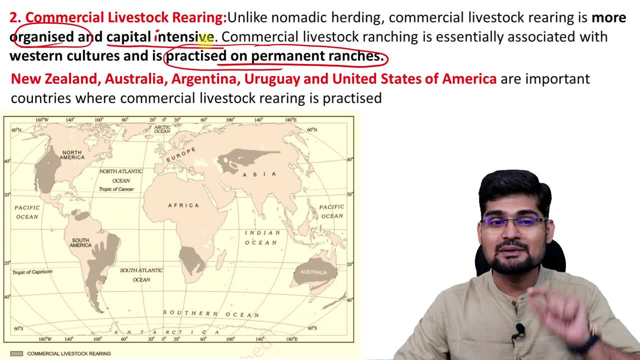 ranches, remember, nomadic herders are not permanent settlers, but this commercial livestock rears are almost permanent in their setting, in their organization. so new zealand, australia, argentina, uruguay, united states of america, the famous countries, you see, they practice this commercial livestock ranching. 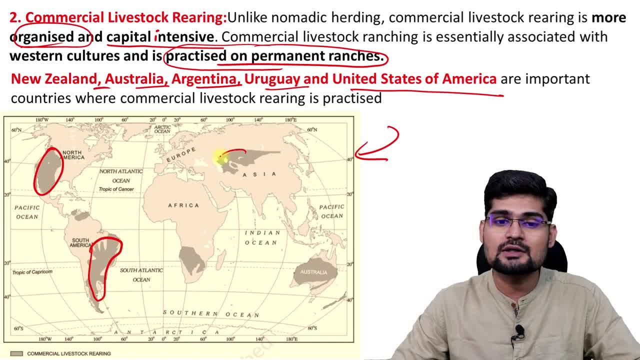 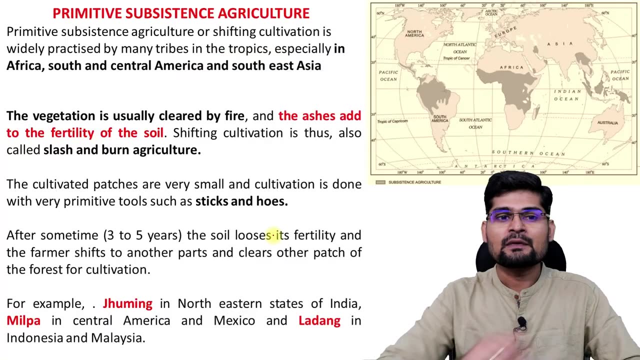 so you see in the map. these maps are very important when you are preparing for civil services examination or for any other examination where you have written answer, for even university exams. so there you can draw such maps and locate the major areas of the world where these kind of activity is found now. 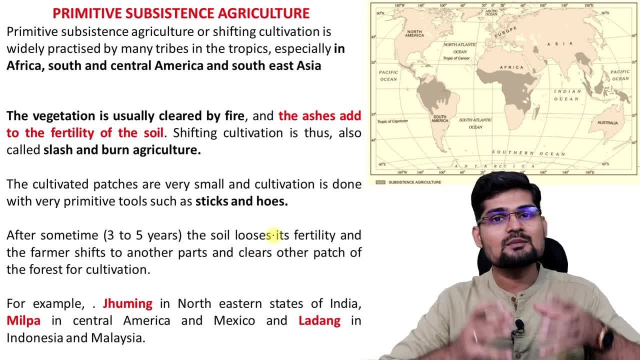 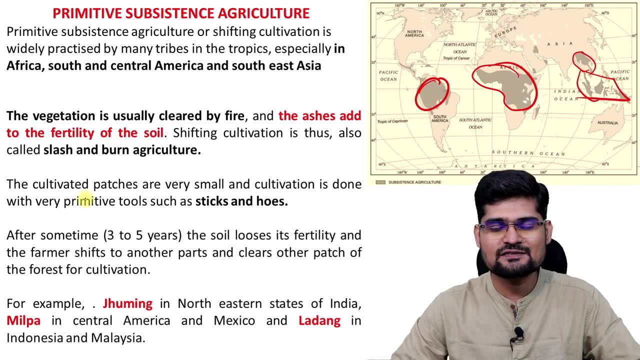 comes the primitive subsistence agriculture. so now comes the agriculture part in which the primitive times, the subsistence was practiced just need based for food right. so you observe again on the map. so the major portions of africa should be the first isiend into pacific america. then you have the indian and south east asia and 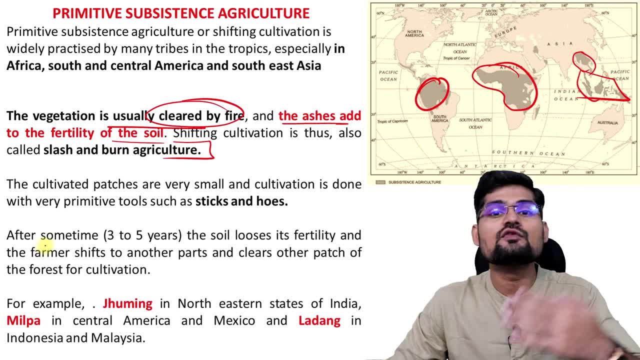 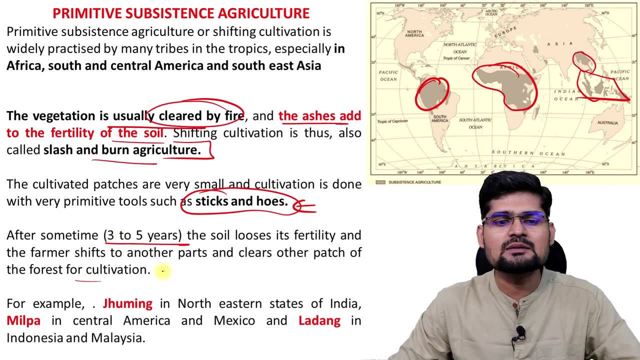 pacific region here on the map. so slash and burn technique. remember the forest used to be cleared by fire and the soil used to be cultivated again when the fertility was lost. other location then to the other location and many times people also return back. farmer shift back. 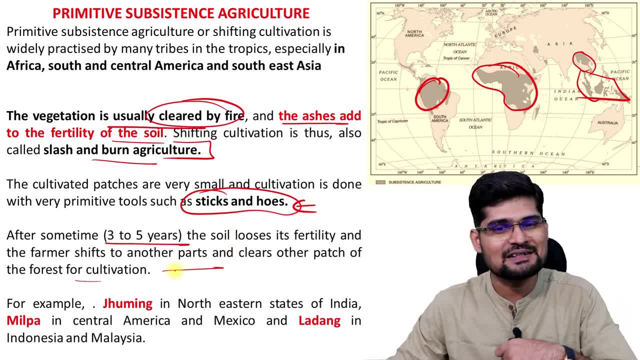 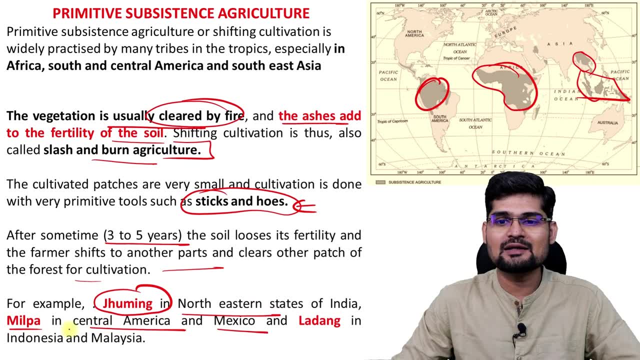 also when they see that the older locations have gained fertility right. so we call this zooming in northeast, zoom cultivation, right, and also milpa. in central america and mexico, this area, it's called milpa, and also ladang in indonesia and malaysia, this region. so that is what you can remember. the 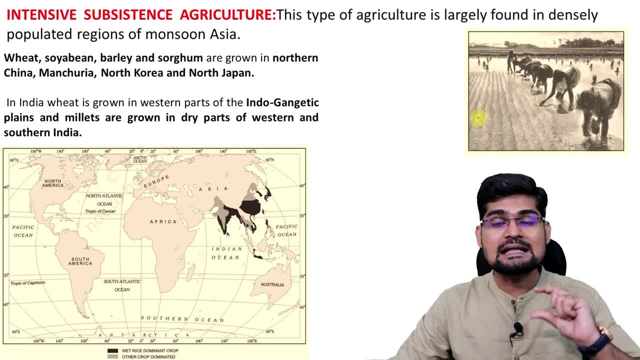 keywords here of primitive subsistence type. then comes intensive subsistence. intensive word itself is intense, too much of input, of labor and also resources, but for subsistence only. so you see this area, this kind of agriculture that we see it's prevalent mostly in south asia, southeast asia. 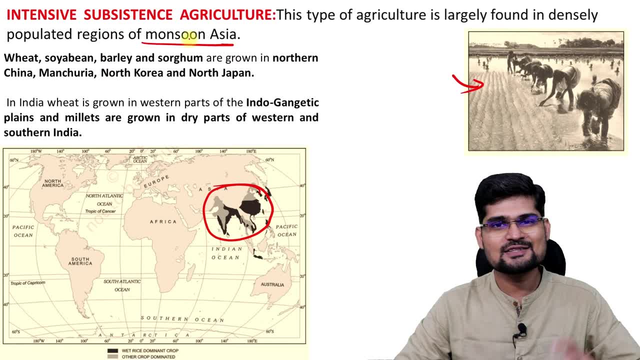 where you have monsoon, asia, right, this you can remember. so what happens here? most of the products like wheat, soybean, barley, sorghum- all these things are grown in china, manchuria, north korea, north japan, and then comes to rice and wheat that is grown indo-gangetic. 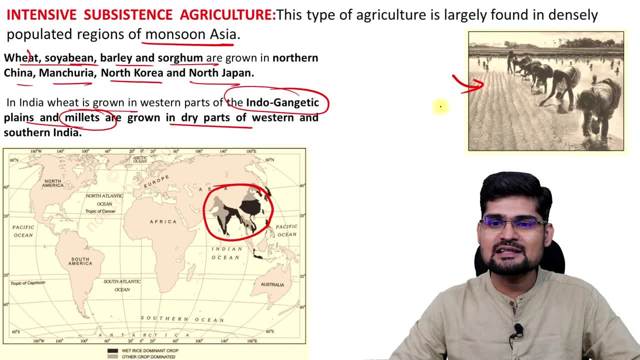 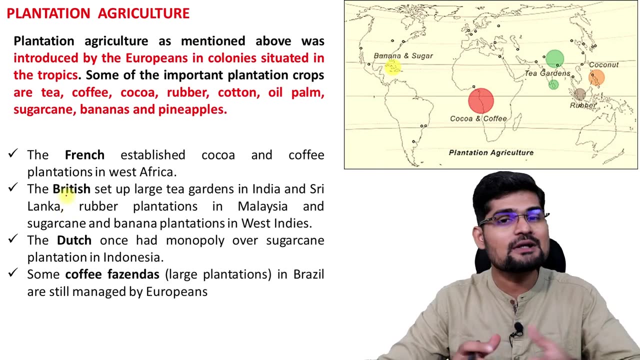 plains. millets are grown in dry areas, so you observe this kind of rice cultivation, wheat cultivation. these are part of intensive subsistence. where you have too much of input of labor, small land holding size, these become important. then comes the plantation agriculture. now, as we know that british popularize this kind of agriculture in their colonies, the european colonies basically. 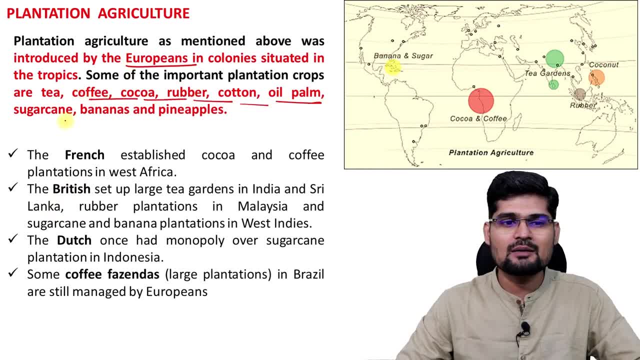 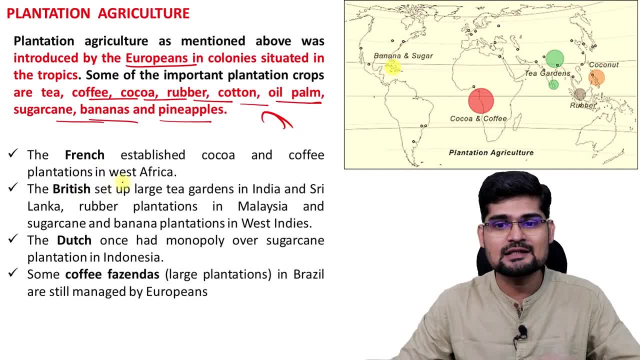 slopes generally right. so this was plantation agriculture in commercial type. if you observe here in the jamaican region banana and sugarcane, cocoa and coffee. in africa, which is west africa segment, then tea gardens and coffee gardens you observe in india and also many coconut and rubber. 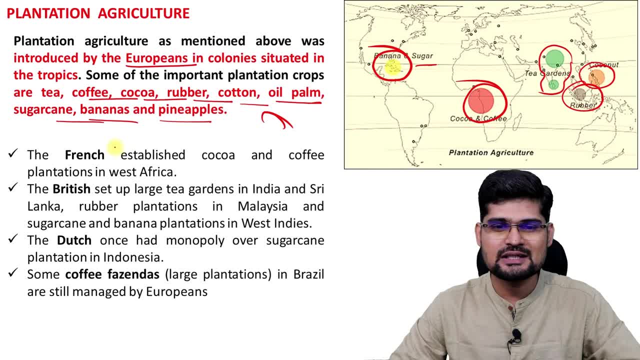 plantations in indo-pacific, southeast asia, indonesia, malaysia. so observe these areas. now comes to the colonies. so you can remember one line about the colonies: french established cocoa and coffee plantations in west africa- this is french colony, then british in sri lanka. rubber plantations in malaysia, sugarcane and banana plantation in west indies. so huge one right. 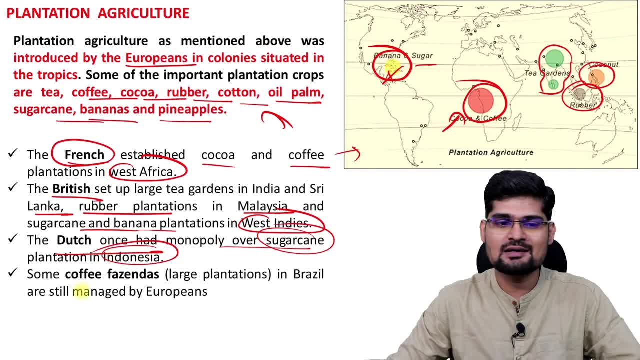 and then dutch monopoly over sugarcane in indonesia and some coffee fazenda. that, we say, is large plantations in brazil. right, this was done by europeans. so this is largely the map of plantation agriculture. so this is largely the map of plantation agriculture. so this is largely the map of plantation agriculture. 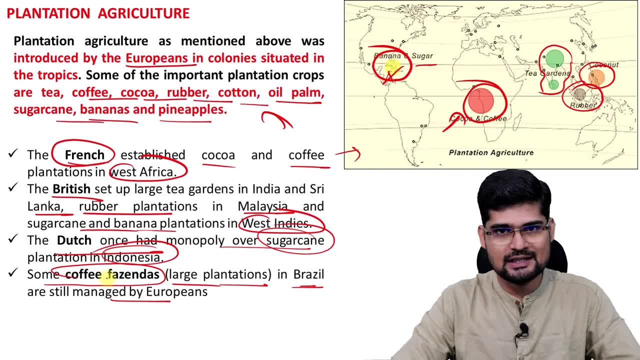 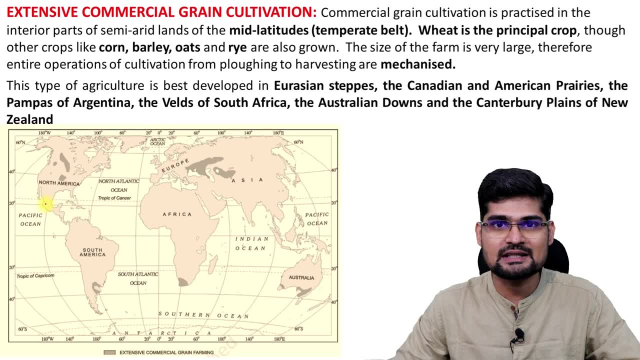 culture which is hugely commercial and colonial in nature. if you observe, then comes the extensive one from the intensive, then we go to the extensive commercial grain cultivation and for this you need what you need: lots of capital and a huge tract of land and technology. this is mostly in temperate. 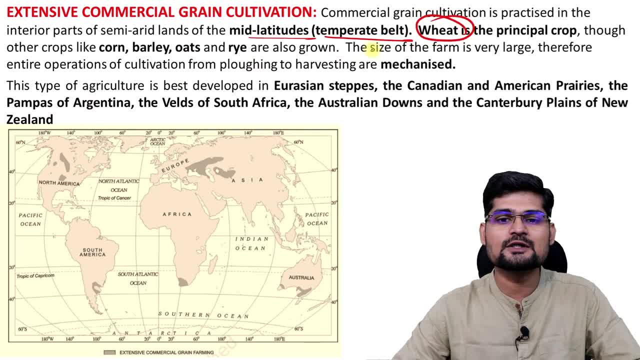 belt, if you observe mid-latitudes, where wheat is the principal crop, and if you observe the us area, then you have some portions in europe and central asia, some portions in different countries, continents, if you observe right so, eurasian stepi, canadian and american prairies, pampas in argentina. 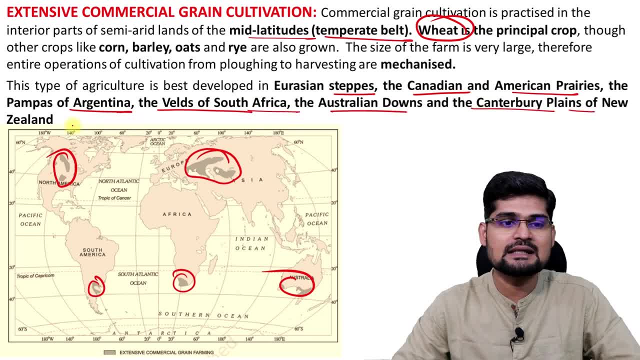 then you have wells in south africa, australian downs and canterbury plains in new zealand. so these are the areas of the world where you have extensive, huge tract of land where wheat is the principal crop, apart from that, corn, barley, oats. right, these are done and this is basically done on. 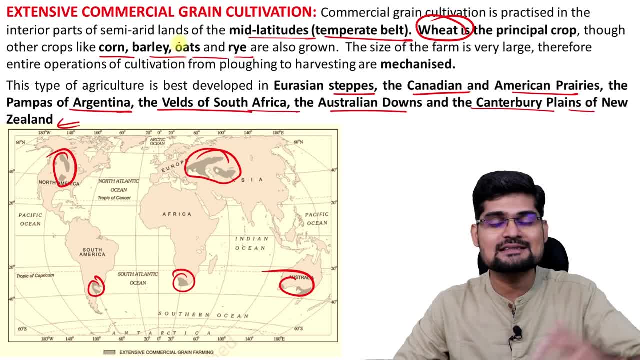 mechanization, basis tractors, threshers for long distances of farming and clearing and again putting the seeds right. so far we have seen that wheat starts to be the principal crop. so far wheat going anything between these are part properly pull at the invested price than i have kids, at least five ahead of last year. 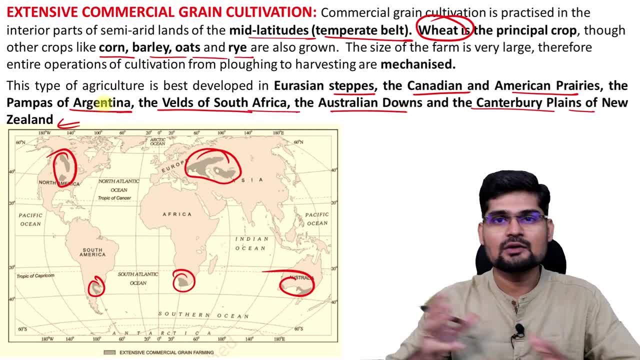 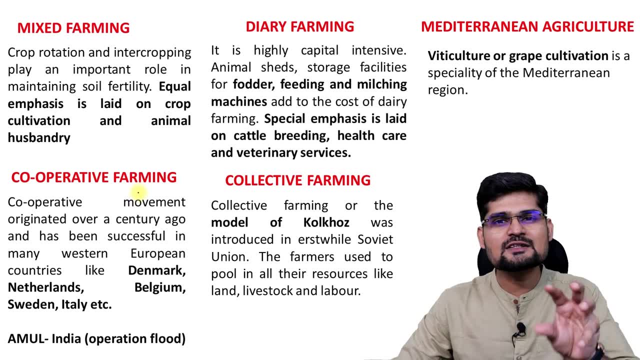 from seed to the last step, that is. you know, harvesting is done in mechanization ways, so that is where extensive commercial farming is. then comes several small, small, small concepts that you can remember. here is mixed farming, where you have equal emphasis on crop as well as animal. 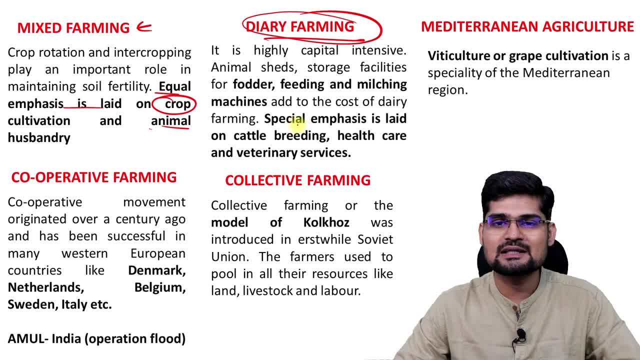 rearing, dairy farming, especially- we know this in india because it's very famous. so what we do? fodder, feeding and milching, so basically milk production comes here: cattle rearing, breeding, health care, veterinary services, including. then you have mediterranean agriculture, the wine production, viticulture, grape cultivation across mediterranean region that we know. then we have 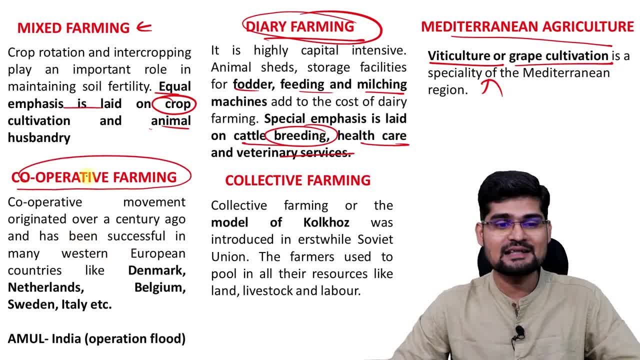 something called cooperative farming as well, which is also primary activity. so cooperative farming is based on cooperation. the word itself is cooperative and it started from european countries like denmark, netherland, belgium, sweden, italy- and remember operation flood in india that is amul, very famous- through cooperative farming. and then collective farming is something which 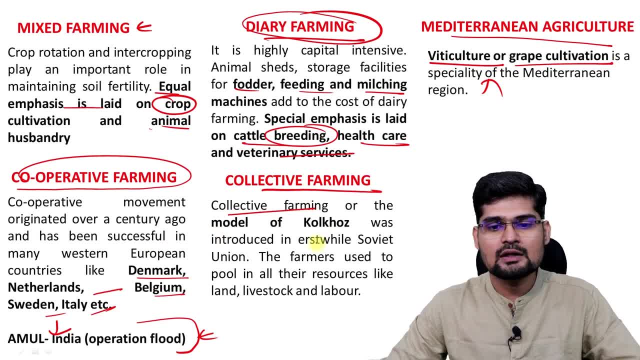 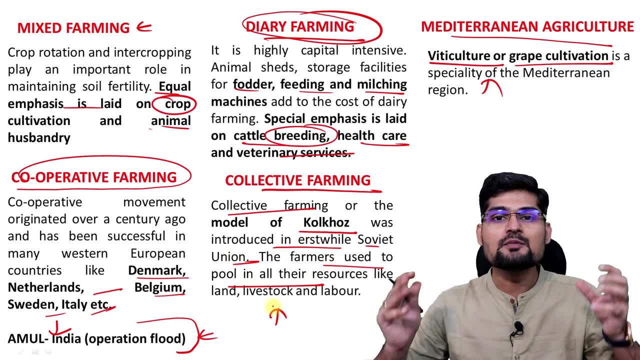 is interesting which is the model of collection called the kolkhoz which was introduced erstwhile soviet union, the russian concept. the farmers used to pool in. so this is kind of a pool in model right. like we have car pool in vehicle pool in, so we have land pool in and also collective farming on the. 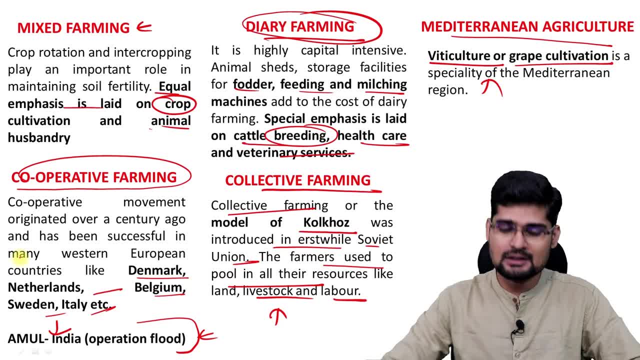 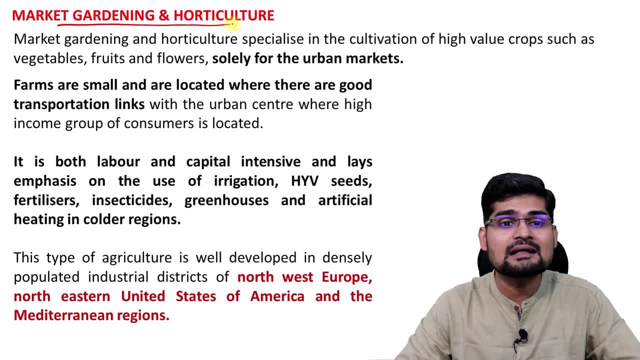 land right, so land, livestock and labor. that's very important. now, after this, we have some two, three more important concepts to learn in agriculture, which is market gardening and horticulture. now, because of right now, we have some two, three more important concepts to learn in agriculture, which is: 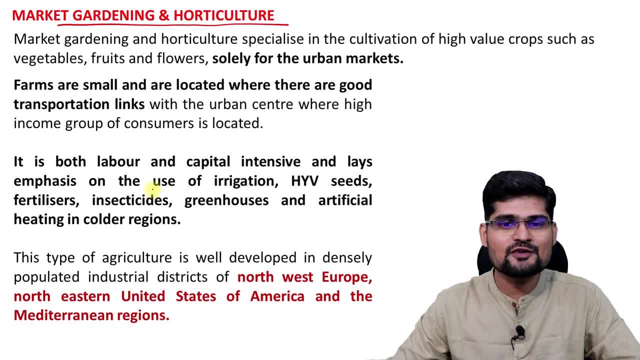 market gardening. now, because of raising urbanization, this has also picked up. so, if you rising urbanization, this has also stolen states. after the start of the world he's hearing, deleting investment and capital was lost to times in the states, right, and so there's also still its housing market, which at this time had been kind in the stars after what like? 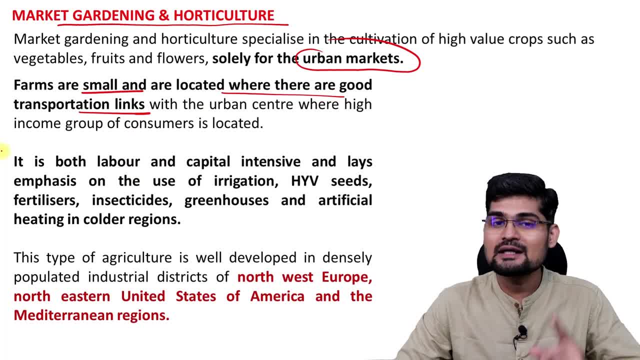 rising urbanization, this has also picked up. so if you observe, this is for urban markets only, for example, floriculture, horticulture, in small areas and grown for the urban use right. so farms are small and located where there are good transportation links. so here, greenhouses, artificial heating in colder region. so if you may have seen in urban areas lot of 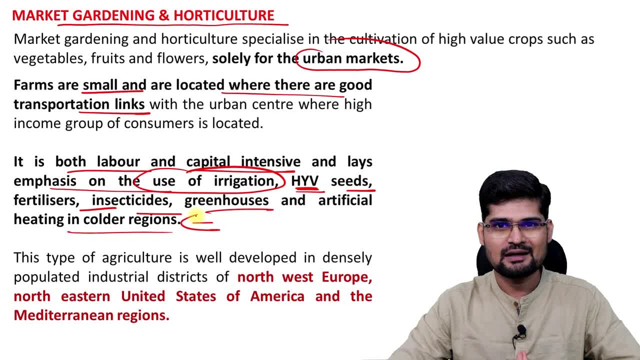 green nurseries and so many growing areas have been built right. they do this floriculture and small crops, and they generally plant vegetables. this is part of market gardening right, so this type of agriculture is well developed in densely populated industrial districts generally, for example, northwestern europe, northeastern united states of america and also mediterranean region. 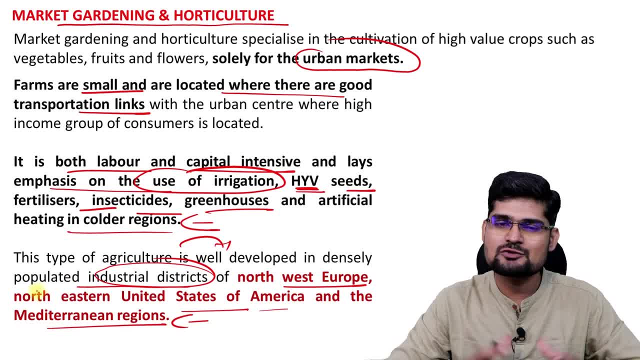 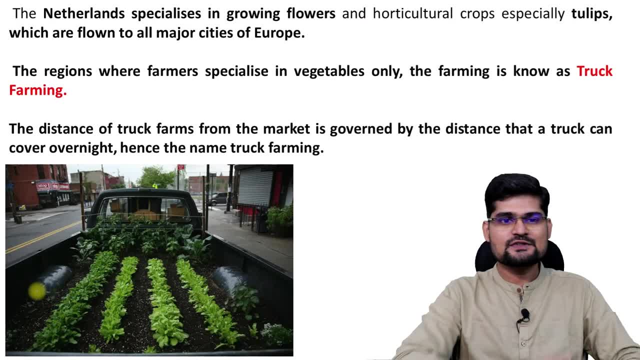 in india also, in urban areas like metropolis, metropolitan region like delhi, mumbai and several others, you can observe this kind of market gardening and horticulture coming up now. so now the point to remember here is: netherlands specializes in growing flowers, right the tulips. 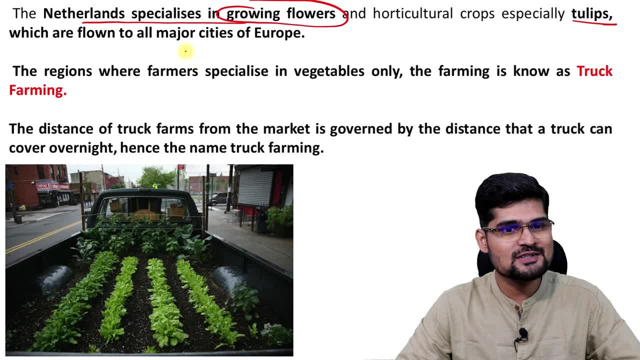 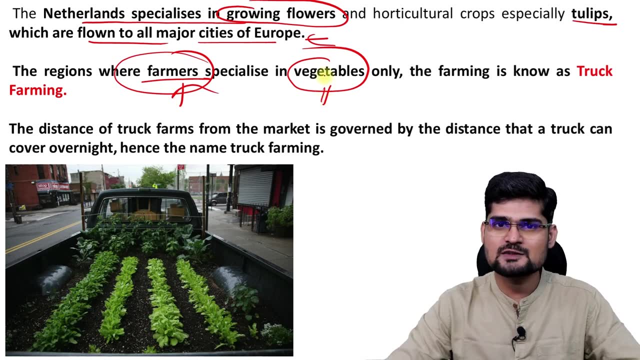 as you remember, and also we have that same in kashmir as well. so flown to all major cities of europe from one place. then regions for where you have farmers specialize in vegetables only. so this is very interesting: that only where farmers grow vegetables and they connect with the roads and transport and supply on the 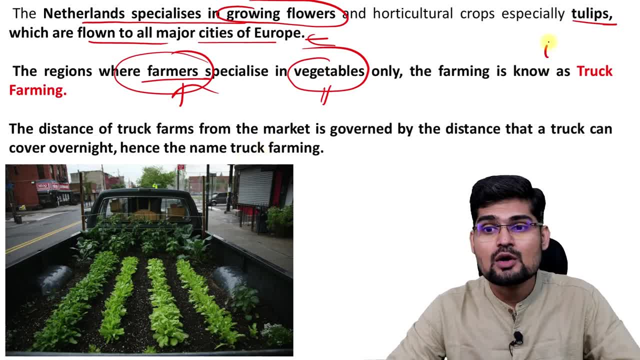 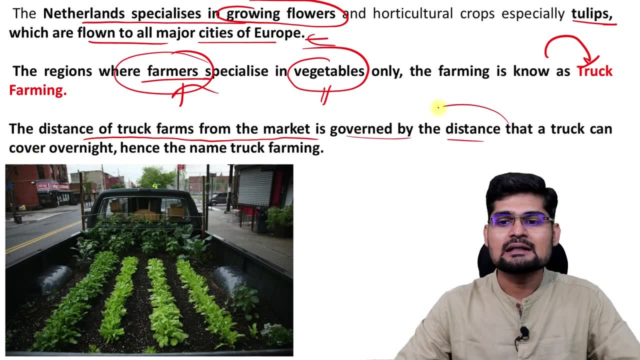 daily basis or weekly basis to the urban areas. it's also called truck farming. why is it called truck farming? because the distance of truck farms from the market is governed by the distance that a truck can cover overnight. so it means it has to be produced, packed and sent overnight. that's done. 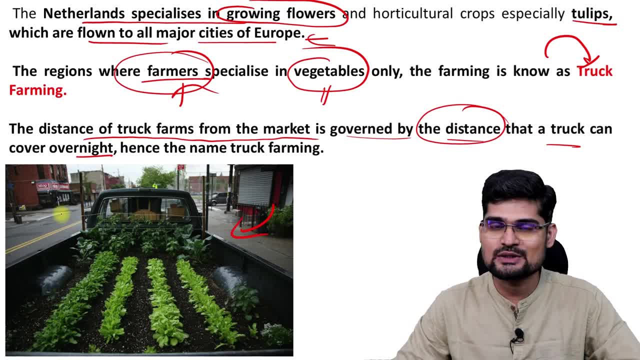 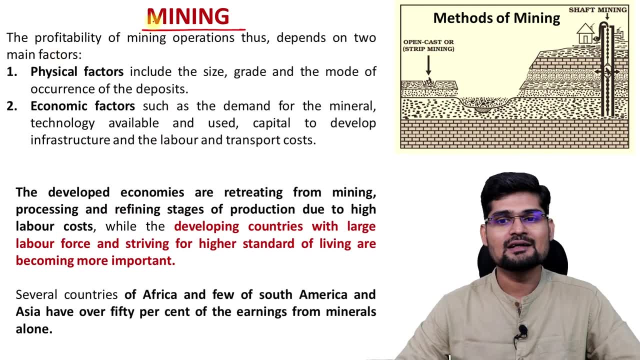 through trucks. so this is how you can see the truck. farming is also done, so it's all based on transport connectivity. now the next activity after agriculture: we have mining activity. so the methods are open cast mine or shaft mining, and this is very common in india, so you can also connect to it. so what are the factors? physical, 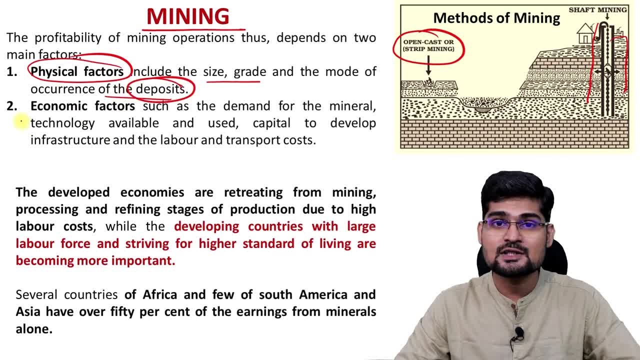 factors like size, grade and mode of occurrence of the deposits, which kind of mines are there- coal mines or other mines- and economic factors, now very important because it's primary economic activity. so the factors, for example, capital to develop the infrastructure, labor, transportation costs, these matter during mining activities. 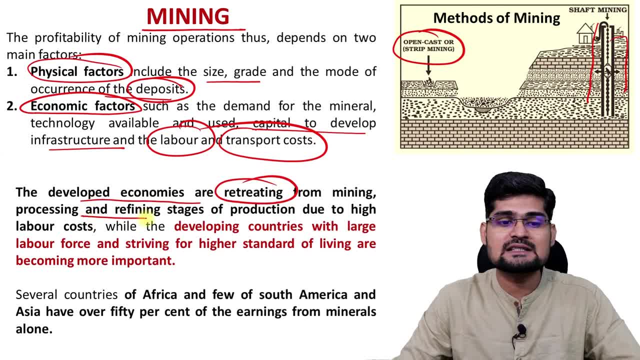 so developed economies are retreating from mining, processing and refining stages of production due to high labor cost. but because of developing countries have lots of population, lots of labor, so cheap labor is available. so still this is dominant activity, right? so several countries of africa, a few of south america and asia have over 50 of earnings from minerals and mining alone. 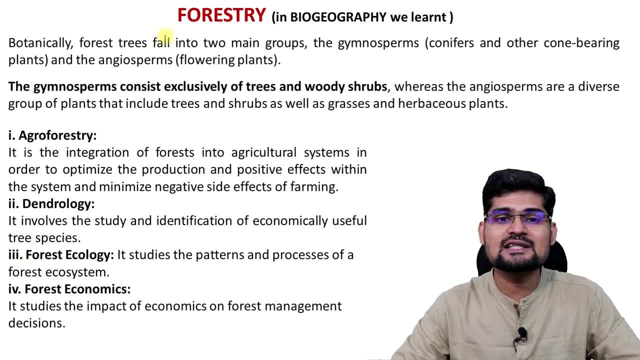 that's very important. now. the next activity that we know is the forestry, and also about it we have learned in biogeography. if you have not watched biogeography videos, you can go there in the playlist and watch it. there we have discussed about forests and other things related to it. 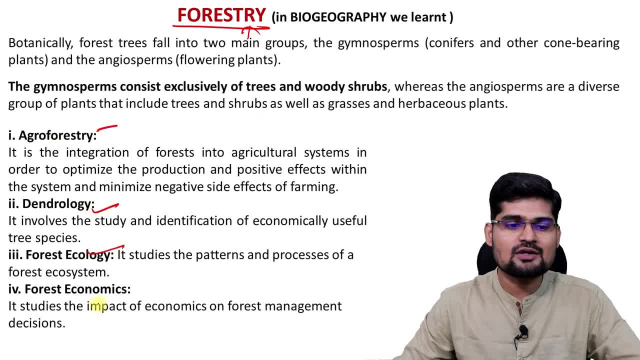 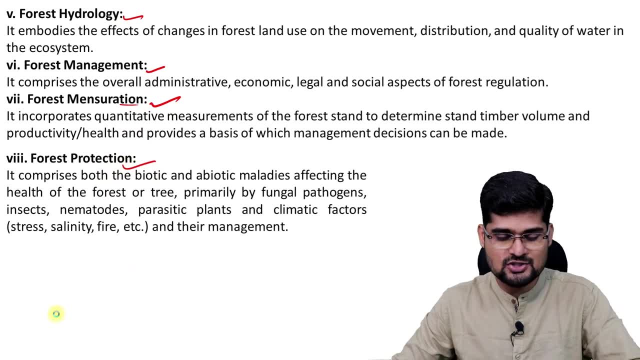 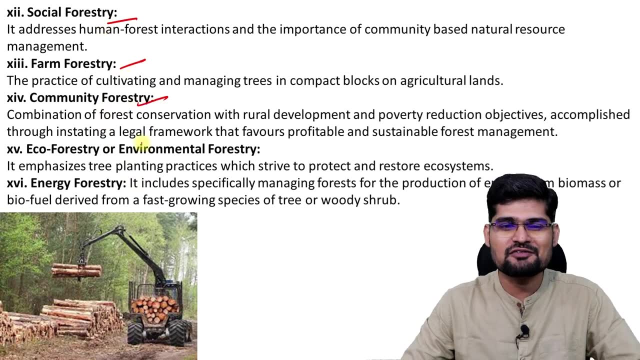 so there agroforestry, dendrology, forest ecology, forest economics, then forest hydrology, forest management, forest mensuration, forest protection, then you have silviculture, tree breeding, urban forestry, then we have social forestry, farm forestry, community forestry, eco forestry or environmental forestry, that we say energy forestry, and then we have agroforestry, and then we have 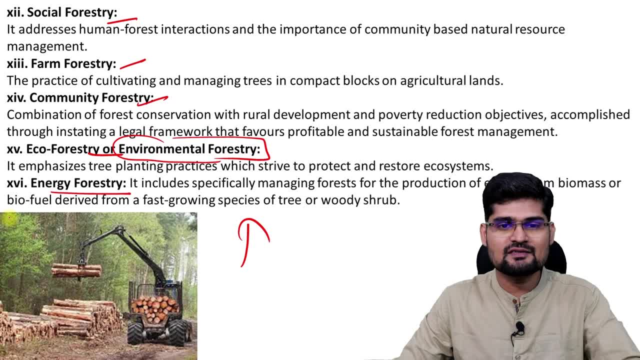 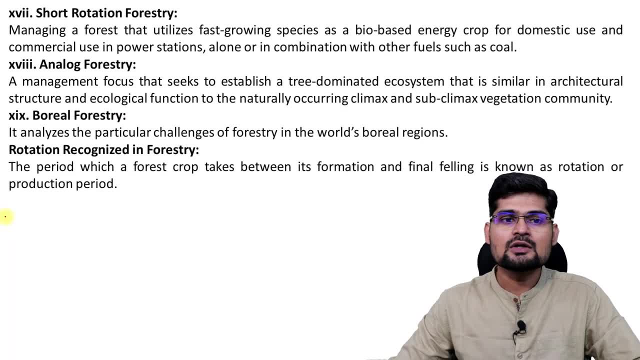 all these things are very important. types of forestries- and i've given this here. you can pause the video and one lines you can study from here that these are the various types of forestries being done now: short rotation forestry, analog forestry, boreal forestry- remember, in the boreal areas of the world- and rotation recognized forestry is also taking up. 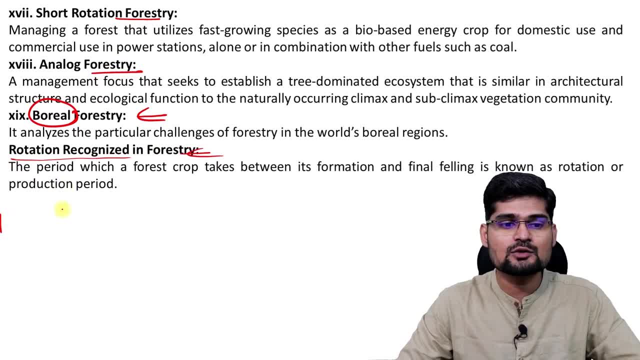 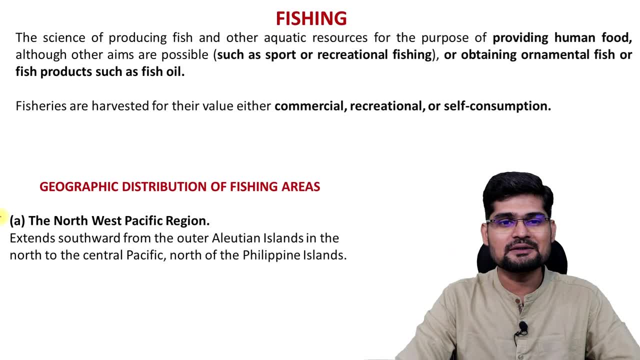 in different portions of the world, so observe almost 19 to 20 varieties of forestries available across the world, and it's essentially a primary activity which is important to learn. then comes fishing. now, coming from India, fishing is really important because we are a peninsular country, right. so the science of producing fish and other aquatic resources, 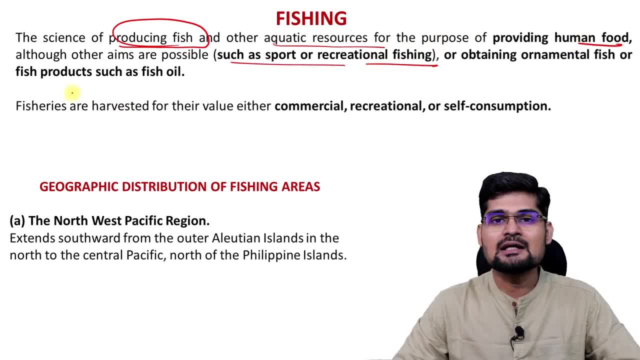 for human food and commerce, and recreation and ornamental purposes also. it's called fishing, as we know, and fishing is done either commercially, for recreational or self-consumption purposes. now look into the different geographic regions where fishing is prominent. one of them is north west pacific. region where you have olesian islands, central pacific and philippine islands. there it's very famous. then comes northeast atlantic and adjacent waters of arctic- very famous areas, right. so what? extending areas from iceland to mediterranean shores. this area includes the scandinavian. 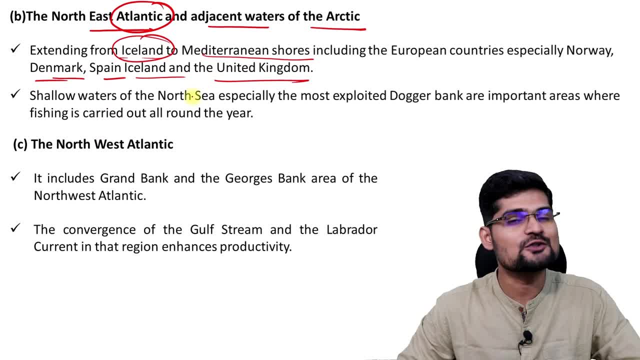 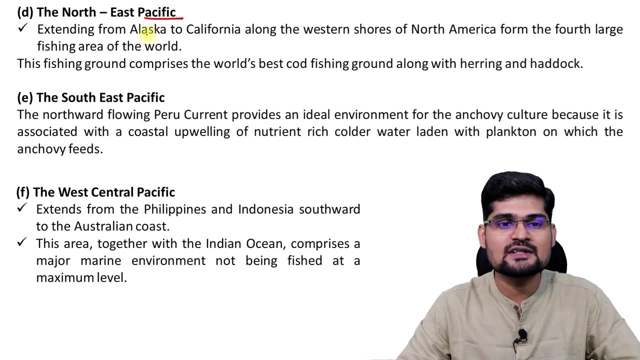 countries: norway, denmark, spain, iceland and also uk. then you have northwest atlantic areas as well, so grand bank and georges bank, right so, where you have gulf stream and labrador current meeting. this area is very famous for fishing and several other activities. then comes northeast pacific. 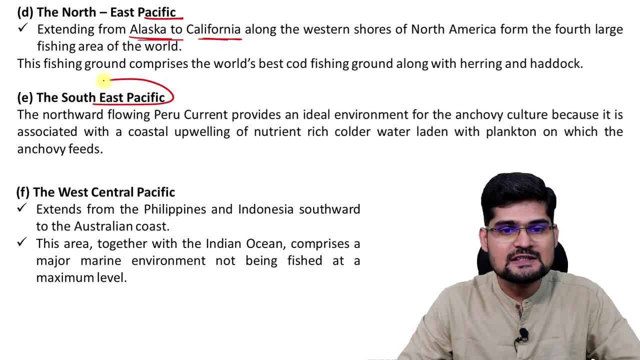 right, extending from alaska to california, then southeast pacific, where you have peru- current- remember it's very important- we have also talked about it in oceanography as well- and then comes the western central pacific, where you have philippines and indonesia, and southward to australian coast. now, when we know these areas, what you need to do is map these areas on the. 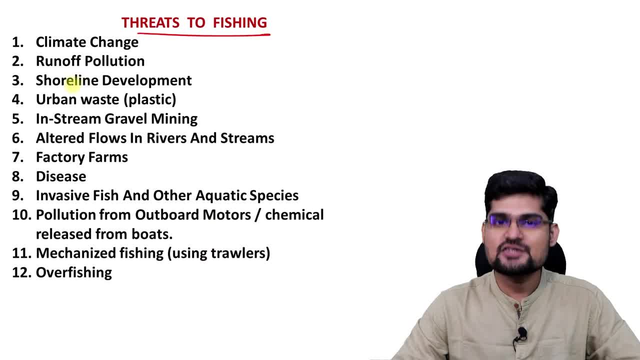 world map right. so what is the threats to fishing activity? if you want to observe quickly? these are the points to remember: climate change, runoff shoreline development, urban waste, plastic waste has been hazardous, in-stream gravel mining, altered flows of river and stream, factory farms, diseases, very common pollution, mechanized fishing over. 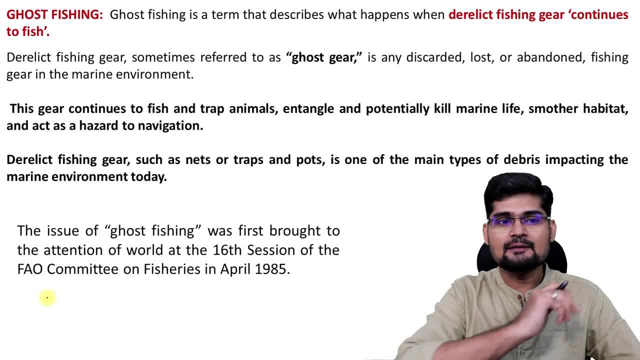 fishing. all these problems are related to the fishing right, and then ghost fishing is one activity we should learn about, because ghost fishing is that when there is a derelict fishing gear used, it means now the fishing gear which is used for the activity- fishing activity is now in bad condition. 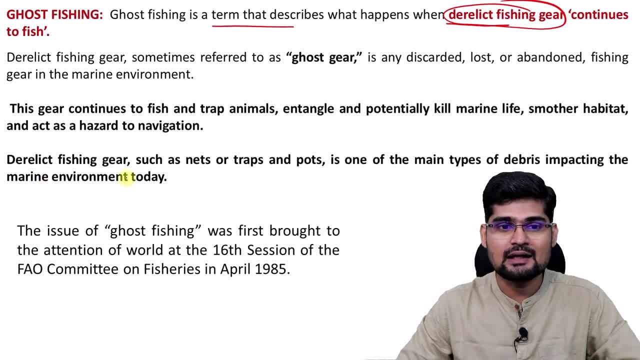 or degraded condition. still, it is being used by people, right, that's also called a ghost gear because it is not discarded. it is again reused, but it should be actually discarded. so this is kind of a thing where ghost fishing is also done in several areas. and remember, ghost fishing is 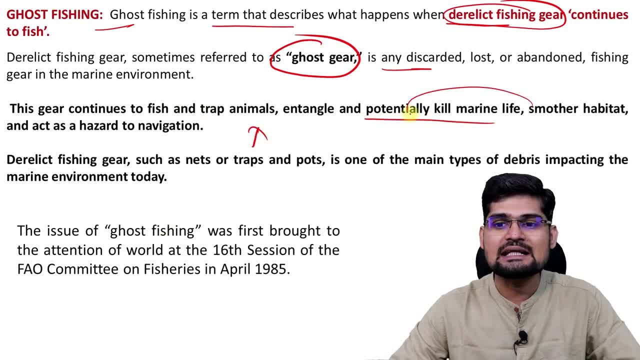 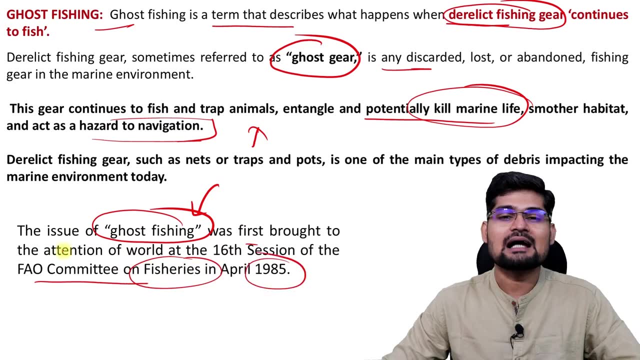 not good for marine life, right? because it is potentially killing the marine life and also changing the habitat and hazard to navigate the marine life. so ghost fishing is not good for marine life, right? so ghost fishing concept becomes important also alongside fishing, because it was first brought by FAO committee on fisheries in 1985 and still prevalent in many areas. because 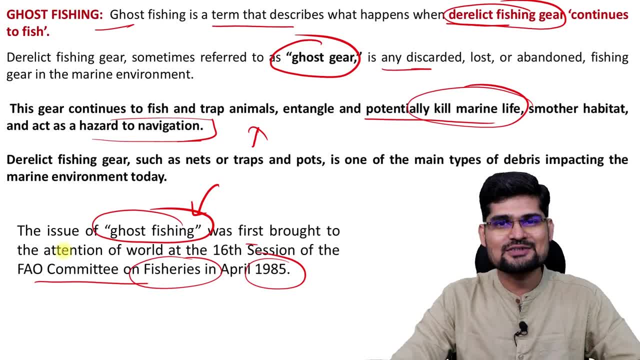 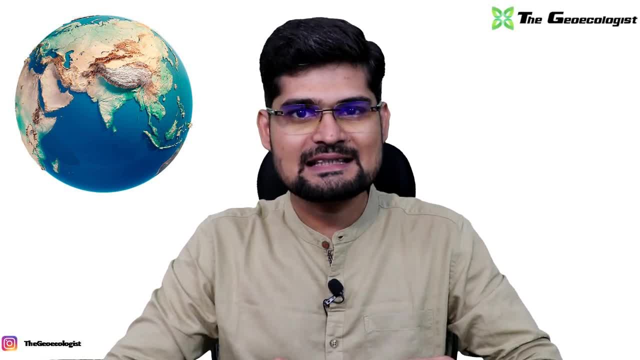 they go against the government norms, right. so this is why it's called ghost fishing as well. so now when we have learned about the different aspects of primary activities in economy, various case studies, examples and distribution across the world, in the sessions to come we'll be talking. 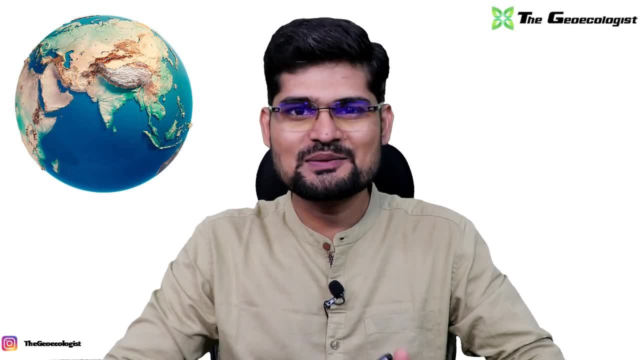 about the secondary activities of the government and the government and the government and the activities in the economy. so stay tuned, stay safe, keep watching, keep learning and don't forget to share the videos with others as well.